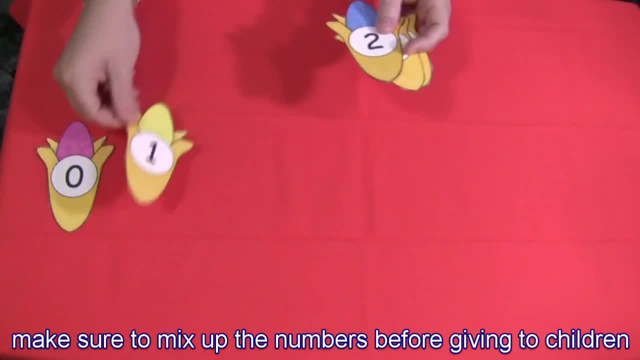 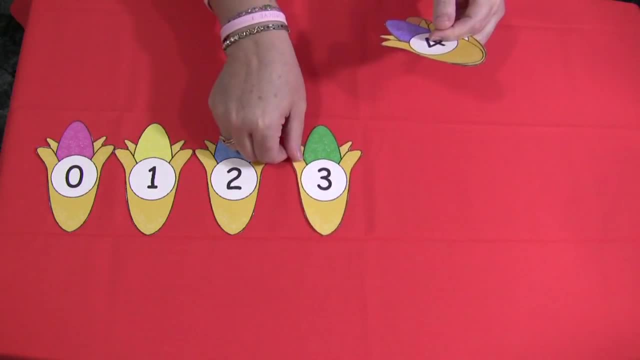 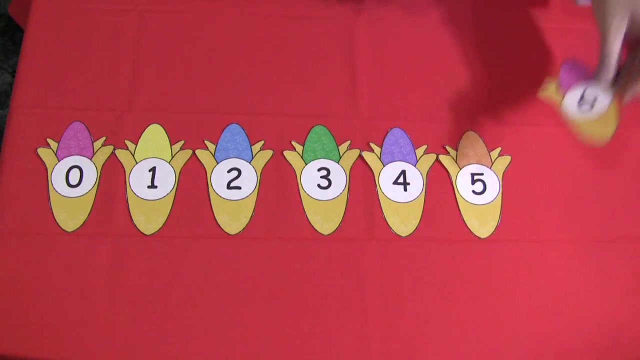 00, 00 put them in order that they would go in numerical order, And again, this depends on the skill level of the children that you're working on. It's a great activity for sequencing and number recognition. Once, because there's a limited space here, obviously I didn't go. 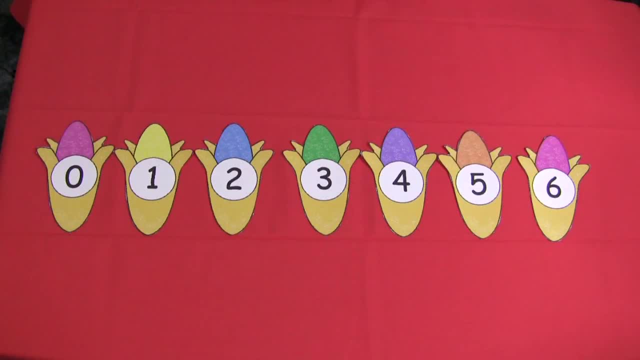 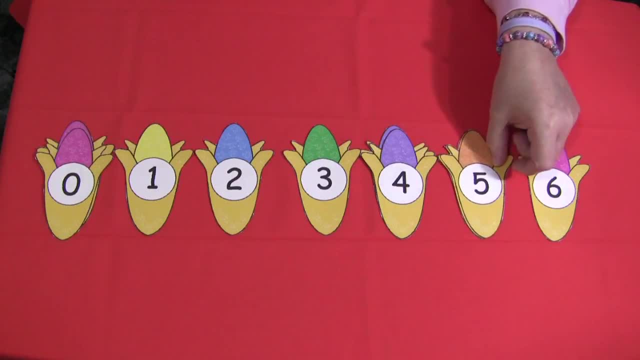 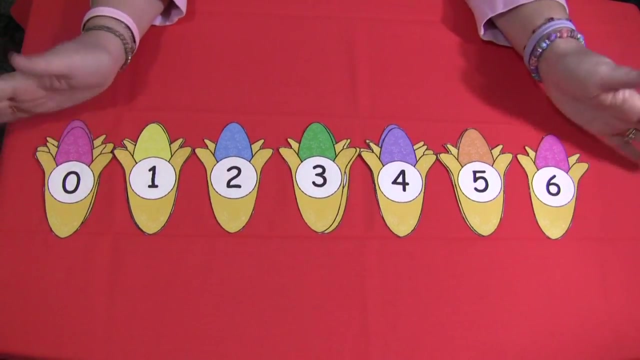 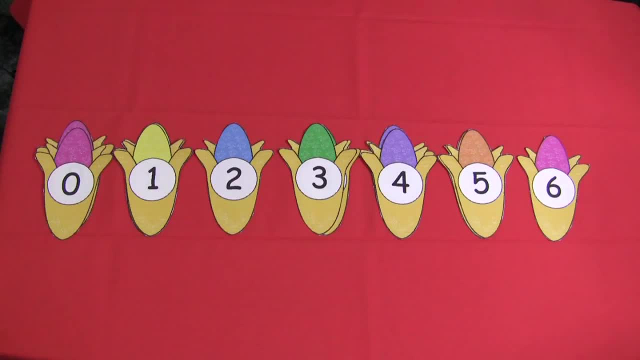 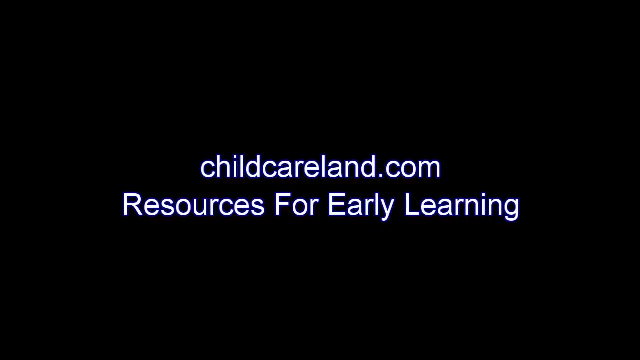